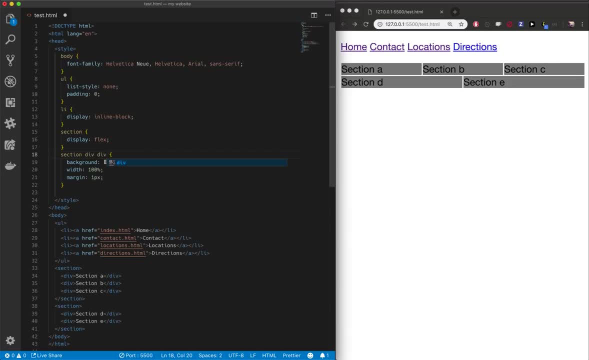 sections. You can keep going here. You can say divs inside of divs that are inside of sections, or u-l-l-i-a. This would be any a that's inside of an li, that's inside of a ul, that's inside of a div. 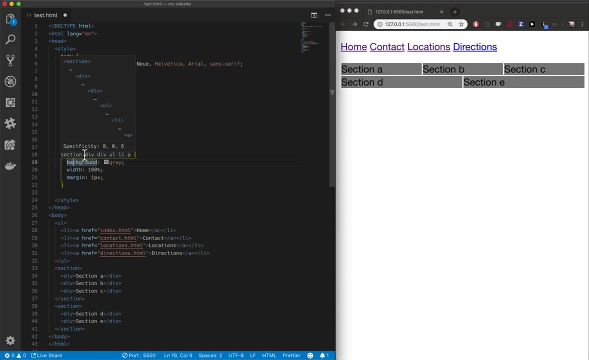 that's in a div, that's in a section. It's a pretty complex rule, but you can go as long as you want. You can also do a comma and say this is going to be a div. You can also do a comma and say this is. 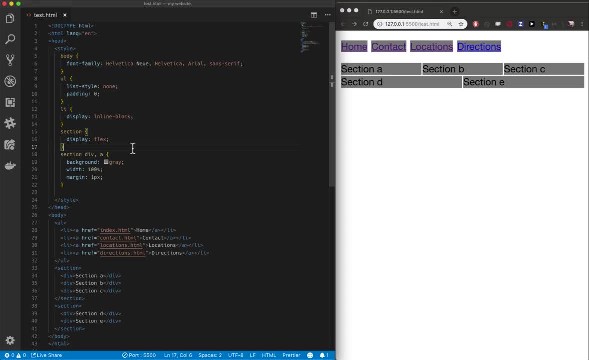 going to apply to more than one selector, But let's say we also want them to apply to any. a tag on the page. So there we go. Now we have a tags on the page. They're also getting the gray background, and any section divs on the page also get the gray background. So you can do commas, You can do as: 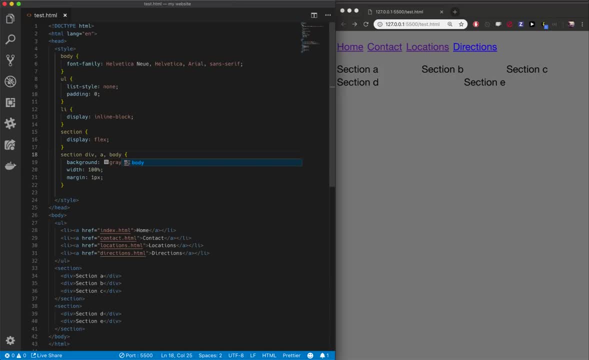 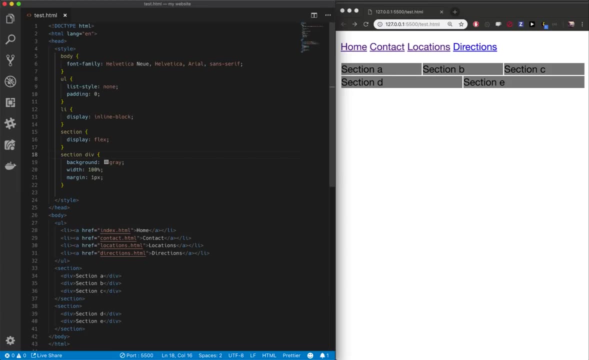 many commas as you want. We can make this apply to the body as well. Now the whole body gets a background color. You get a background color, You get a background color. So that's kind of how the commas work. Spaces and commas- That's your basic selector rules, as you can add spaces to say: look. 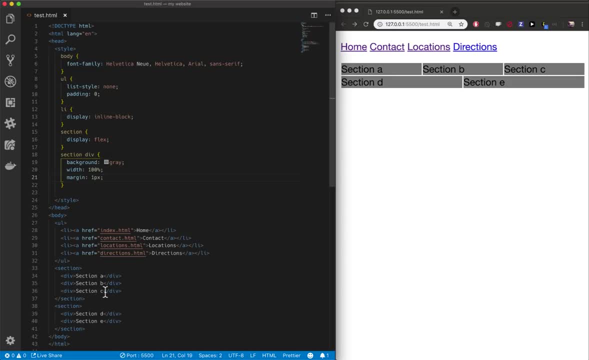 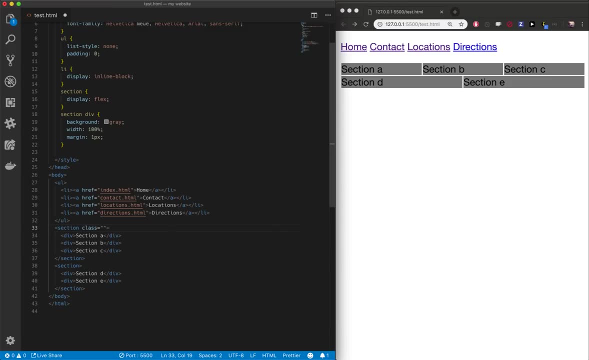 and you can add commas to say, oh, we're going to do this as well. So let's look back to the class problem. What you can do down here is you can add classes to your html. class equals and then anything inside of here is a class. Let's give this class, let's call it a feature box. You can't. 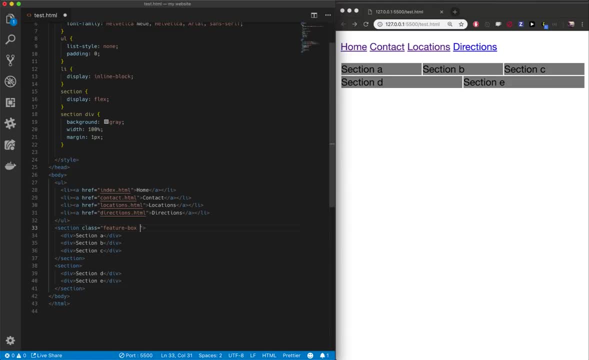 use spaces in your class names, because whenever you use a space, you're giving it a second class as well. So this will be: this: will have two classes, feature box and we'll call this sales. You can add it. You can add it before You can add it. before You can add it. before You can add it. 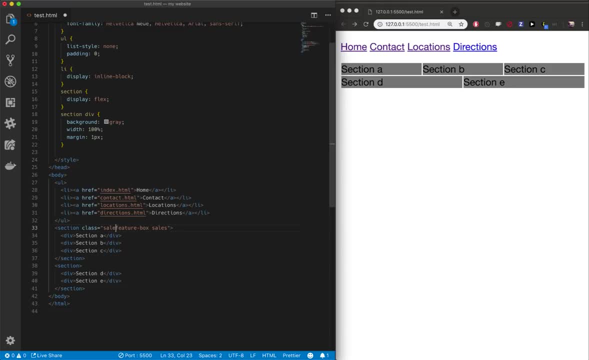 sales here: Sales space, feature box or feature box space sales. It does not matter. Whenever you add a space, you're adding a second class, and you'll see what that means here in just a moment. Let's give this one here a class. This will also be a feature box, but this one will be closeouts. 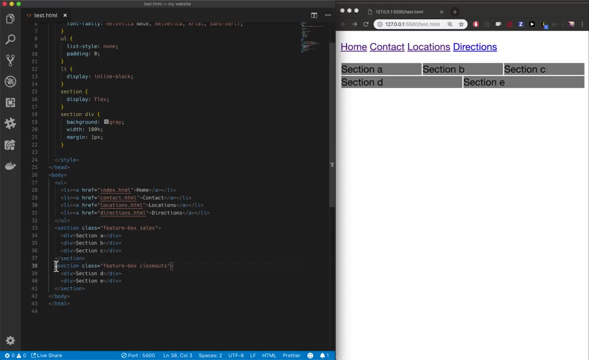 So we have two feature boxes, Our sales feature box and our closeouts feature box, and now we can target them. So we can say: let's go up here section dot, feature box. this is any section with a feature box class inside of it Doesn't matter if the feature box class is second or first, if it has a feature box class. 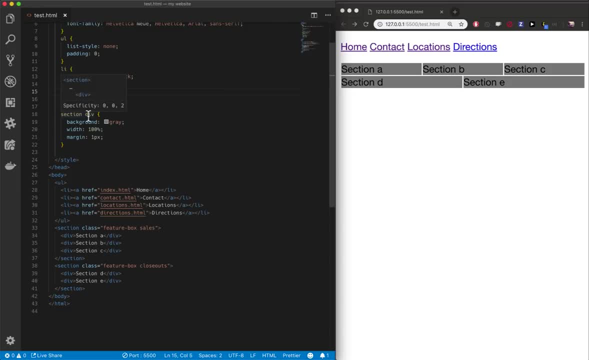 it's going to get this rule. and then also you can say: any section, feature box, div gets these rules, so nothing changed, because we're still targeting this section and this section. But now we can do: here is feature box, dot sales, we're going to only target. 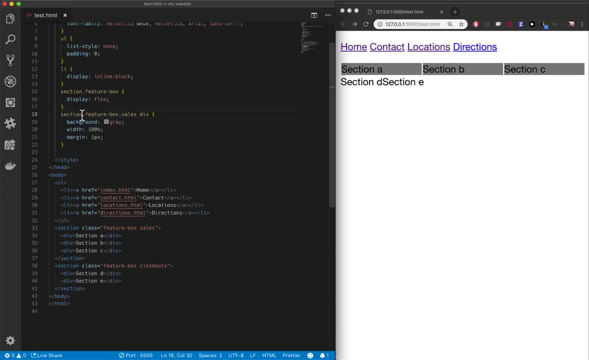 have the class feature box and the class sales. you'll notice i did not add spaces here. space would say: let's look inside of section for any element with a class of feature box and sales. we don't want that. we want only section elements with a class of feature box and sales. we want these. 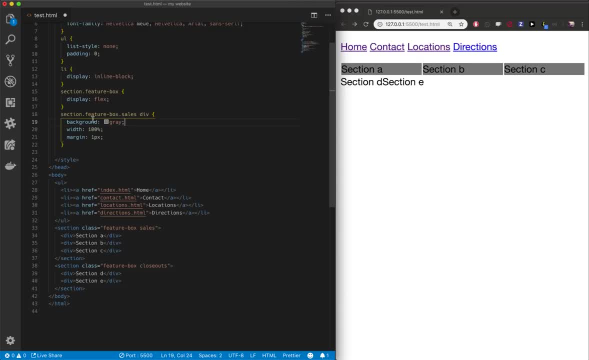 dots to apply to the section element so we connect them to it. so now you notice that only the first one caught those rules. all of them up here. every section feature box is display flex, but only the ones that are feature box sales get that background color. so now i can kind of copy and paste and let's 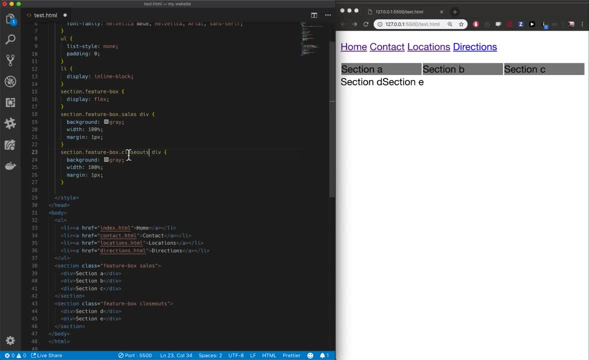 say, feature box closeouts, they're going to get a background color of red, and boom, we've solved our problem. another thing, though, is we've actually copied some code. there's this rule in web development: d r y dry, don't repeat yourself. you'll hear people say: i need to dry this code up. 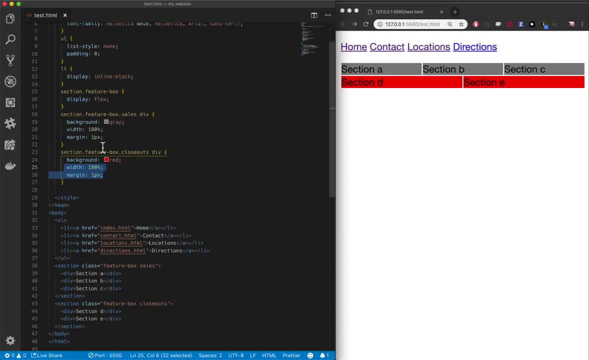 that means that we're copying and pasting some things here that we have to maintain. what if we want to change this margin to two pixels? well, now we have to find every place where we set our margin to one pixel and we have to change it. that's not good. we need to dry this code up to dry this code. 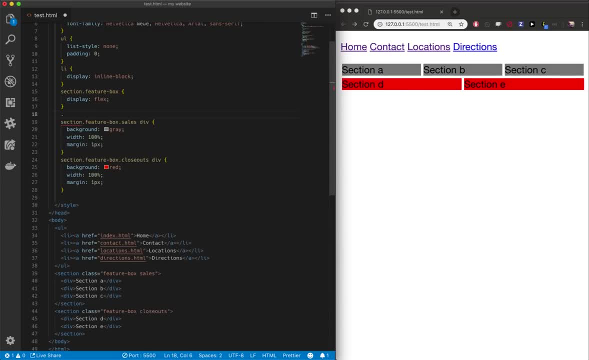 up. it's pretty simple. let's just say: every dot feature box div, every dot feature box div will get these two rules: boom, and then only the sales divs and the closeouts are going to be the same. divs get the rule, the color specified. so that's going to do the exact same thing, but it's drier. 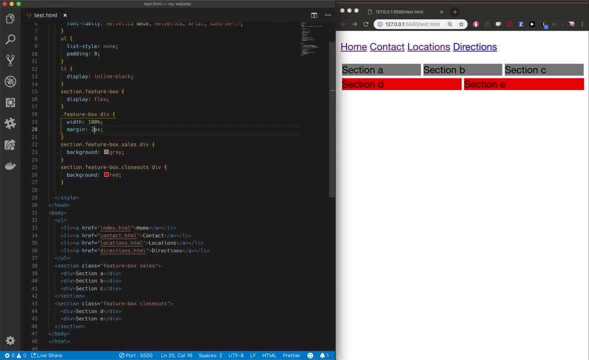 now, if i want to change the margin to two pixels, i only do it in one place, and while it's not a big deal right here, it's so easy to get your code copied to where this little margin- one pixel- is in a hundred different places of your website. you don't know where it is. another way we can clean: 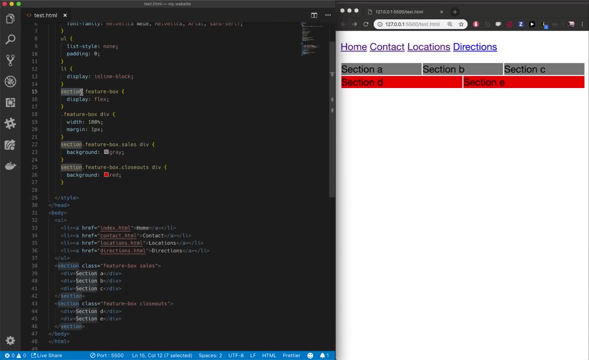 this up is we no longer have to specify section here because dot feature box does it all. there's not any other places on our website that are going to have dot feature box in them, unless we want dot feature box. so we can get rid of the section and look our code kind of reads a little easier. 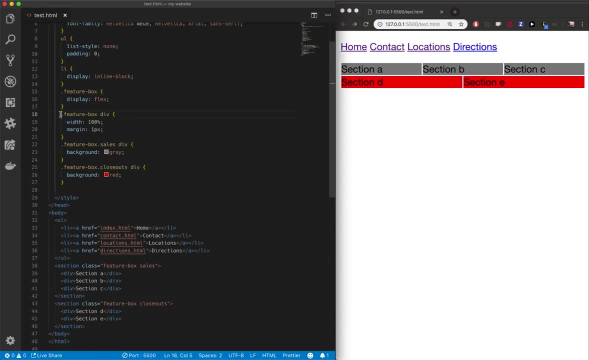 now too. feature boxes: get display. flex any divs inside of feature boxes, get this kind of layout and specific feature boxes have different background colors. that's how you target with classes, classes- you can have as many of any of them on a page as you want. the other way that. 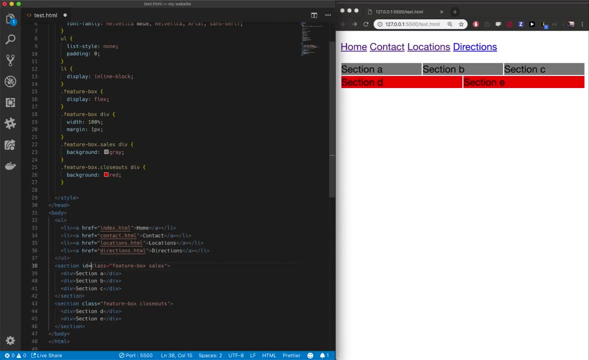 you can target is with ids. ids get id equals and we could give it something. let's call it frank, id frank. you target that by saying pound frank. so anything with id frank. let's give it a font size, a 200 font size. uh, the problem with ids is you can only have one of this id on the entire page. 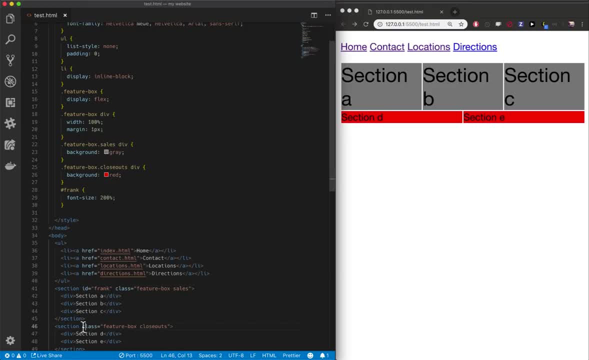 doesn't matter. if you add another id frank down here, that is illegal html- it might work fine. yep, you can see google chrome actually handles it okay, but you don't know what you're going to get on different browsers and different devices, because that's technically the only way you're going to get. 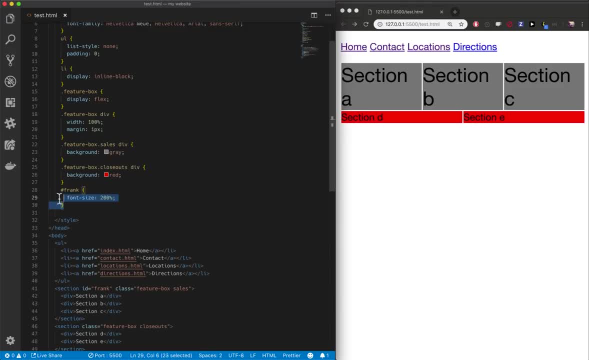 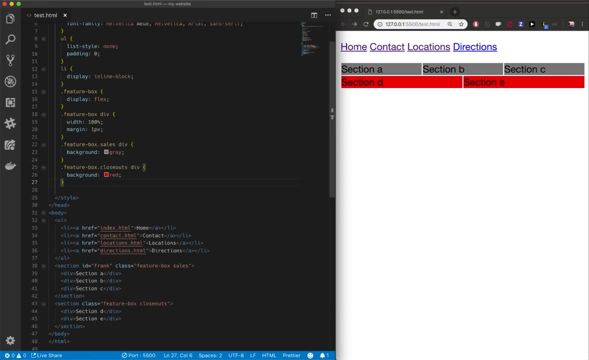 something that's technically illegal html. so ids: usually you can get by by doing class names. you don't really have to do ids stay away from, unless you find a really good reason why you need to do ids. but classes pretty much will always get the job done just fine. so that's how you use class. 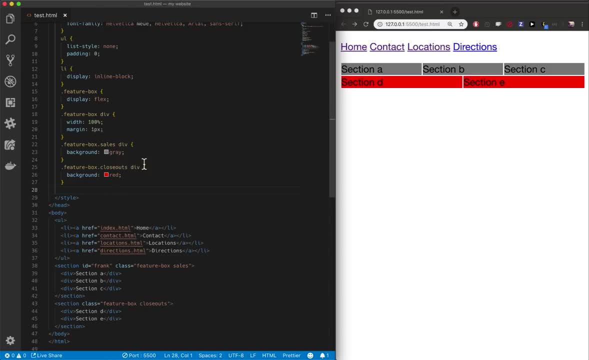 names to specify certain things, and again you can use comma and do a whole bunch of other specific things. we want feature box closeouts to be read. uh, we also want, i don't know, non-feature box- is that a thing? probably not- non-feature box dot closeouts to be read, basically anything closeout. 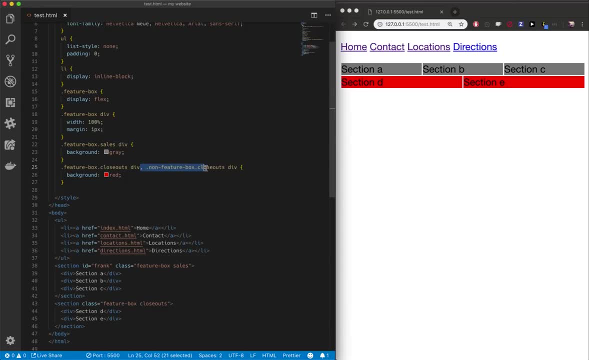 divs. we want them to be read so you can add commas and target multiple things on your page. i'll leave you with one more thing. there's- there's a decent bit more that you'll learn ongoing with css selectors. you don't have to know it all now to become a web developer. so one more thing that i 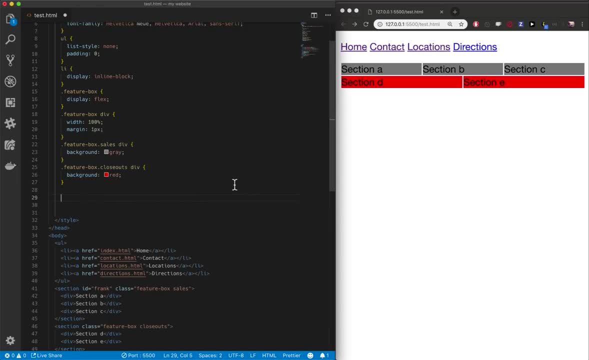 will show you is that the web page provides you things that are called pseudo classes, p-s-e-u-d-o, which means kind of pretend classes. so pseudo classes are things that are called pseudo classes. uh, this one would get a pseudo class of first child. this would get a pseudo class of last child. 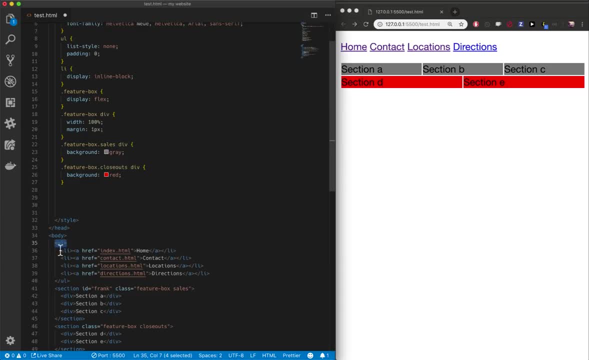 first child means that if this is a parent element, the first element in there is a first child- that's this li right here- and the last one inside of that parent element is the last child. so i could target all first child lis, which is just this home one, and give it a special background color. 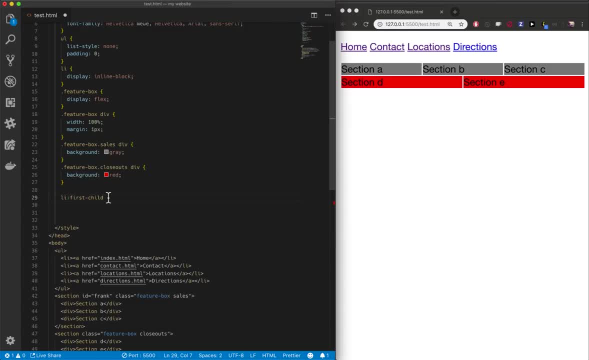 i do that by doing a colon. colon means i'm looking for pseudo class. there's some pseudo classes, provided let's give this one a background color of red. boom, you can see, my first child got a background of red. if i change this to last child, then i last child got a background of red. 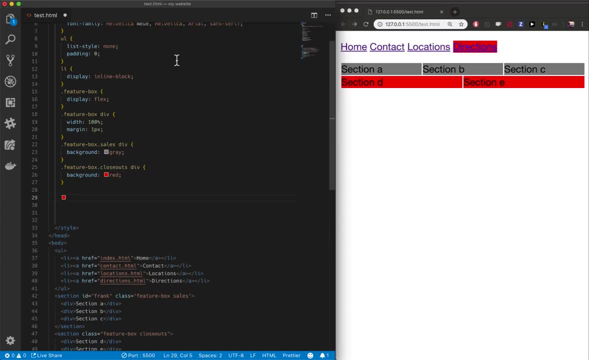 where this is useful is when i want to do some things like, hey, let's uh, give these things a background color, let's give them all a background color of gray, let's give them rounded corners. so now they're doing that. oh well, 10 pixels, that's huge. what on earth was i thinking? let's. 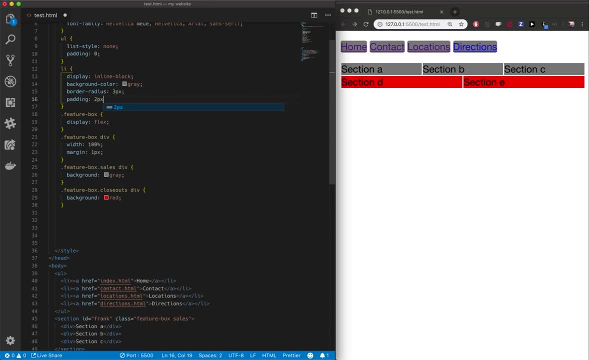 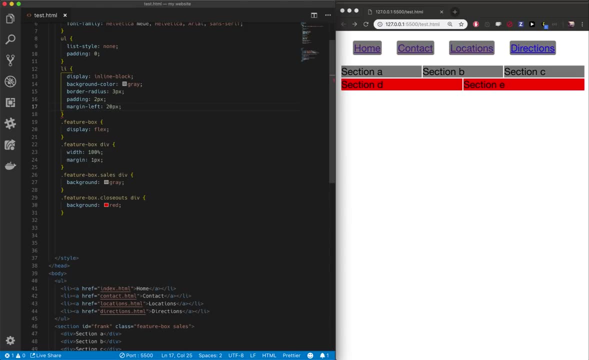 try three pixels, let's give them some padding. uh, let's go ahead, give them some spacing. margin left of 20 pixels. they're kind of spread out a little bit, ah, but i don't want this first child to be bumped over, and that's where first child comes in. 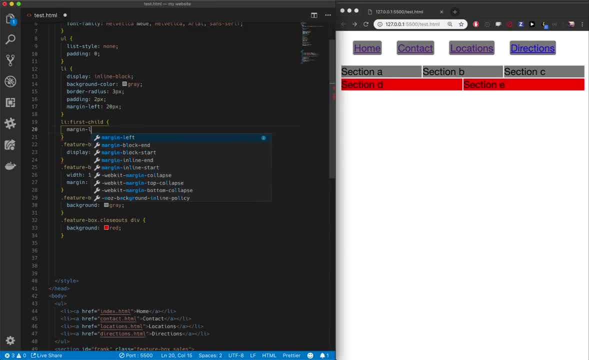 first child will have a margin left of zero, and now it bumps over and i've got the spacing carried out. this is like the ugliest navigation of all time. thank you very much. i'll be here all week, but it gets the point across. sometimes you only want to mess with the first child in your layout in order to keep your layout looking the 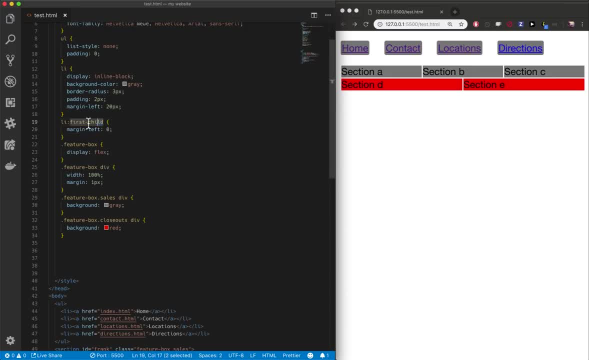 way that you desire. so first child is out there. there's also ones that are active. active this is if your link is active right now. so if i'm on the home page, i can make this home page not be underlined. i could say a colon active that's going to get text decoration.